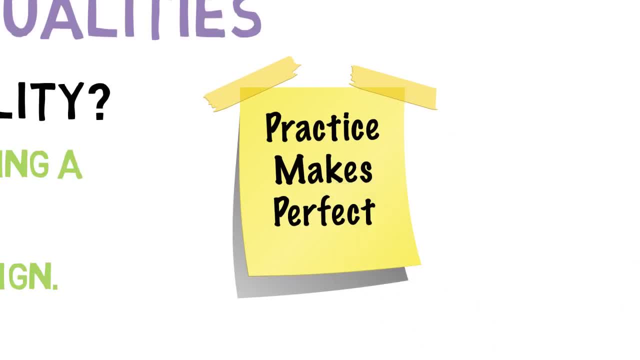 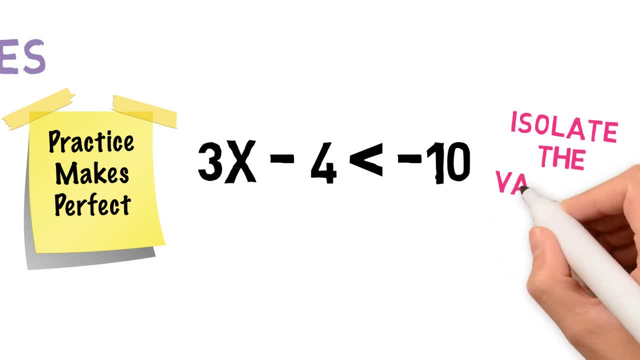 difference between an equation and an inequality. let's practice solving one. Take the inequality: 3x minus 4 is less than negative 10.. Like when solving equations, we want to isolate the unknown variable. This means we need to figure out what possible values. 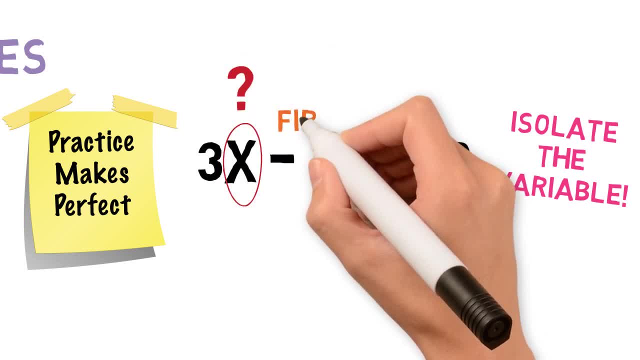 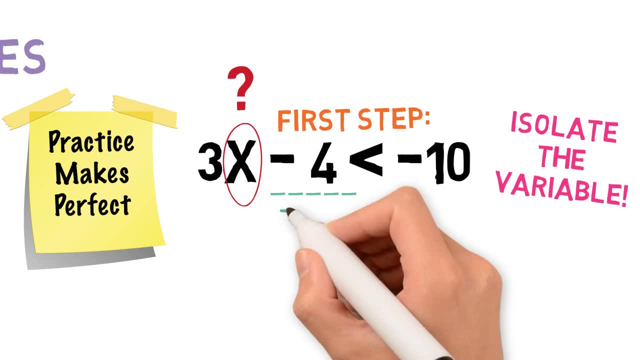 x can be to make this inequality true. So first step is removing the value that is not attached to the variable. In this example, that number is 4.. Since 4 is being subtracted from 3x, we have to add 4 to create a zero pair. After we add 4 to one side, we have to keep the inequality balanced. 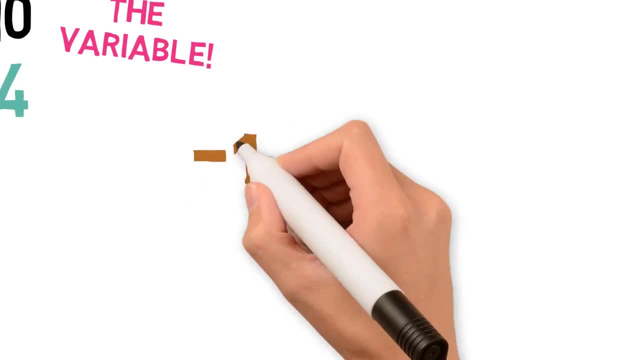 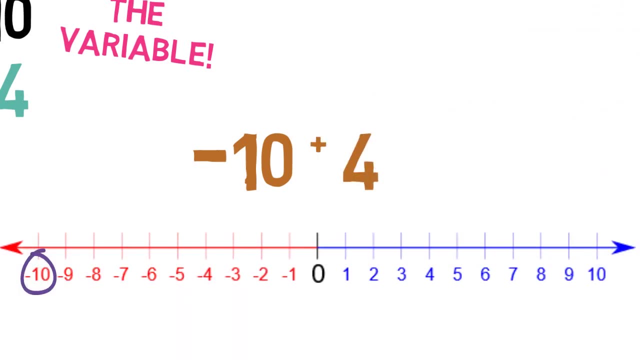 and add 4 to the other side. Negative 10 plus 4 is taking a negative number and moving it closer to 0. Think about a number line. Negative 10 is over here. When we add a positive number to a negative, we are moving to the right, we're closer to 0. So negative 10 plus 1,, 2,, 3,, 4 lands. 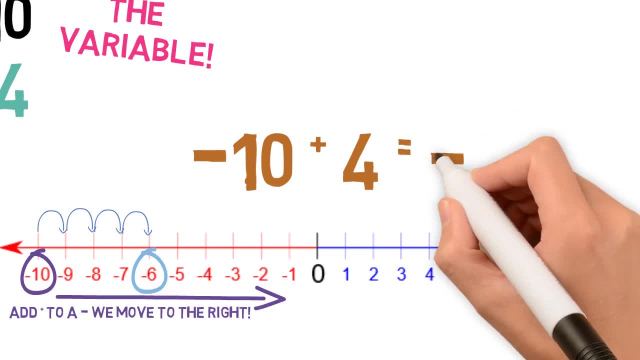 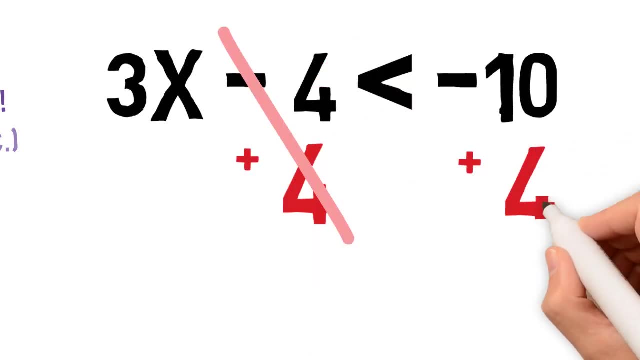 us on negative 6, meaning negative 10 plus 4 equals negative 6.. Back to our inequality. We added 4 to both sides. This leaves me with 3x on the left and negative 6 on the right. We bring 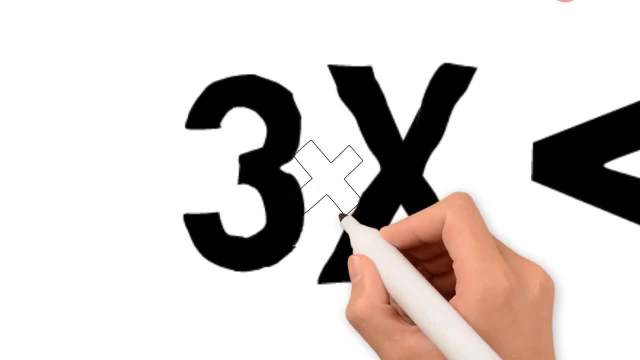 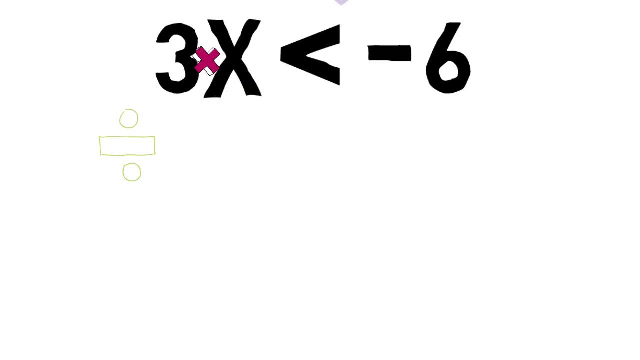 negative 6 to the left and negative 6 to the right. Since x is being multiplied by 3, I need to perform the inverse operation. The opposite of multiplication is division. so I need to divide 3x by 3.. This leaves me with 1x. What I do to the one side, I have to do to the other. so I take 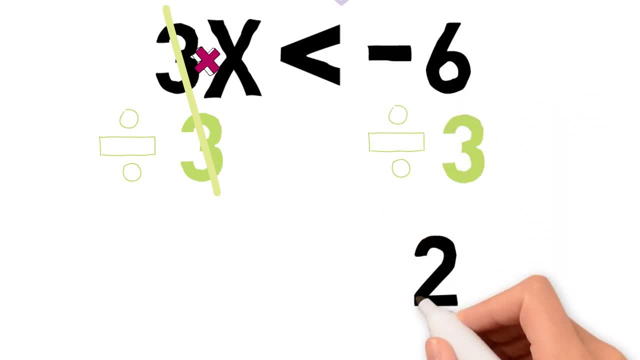 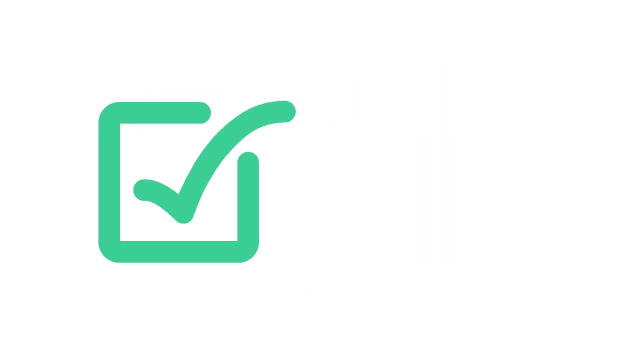 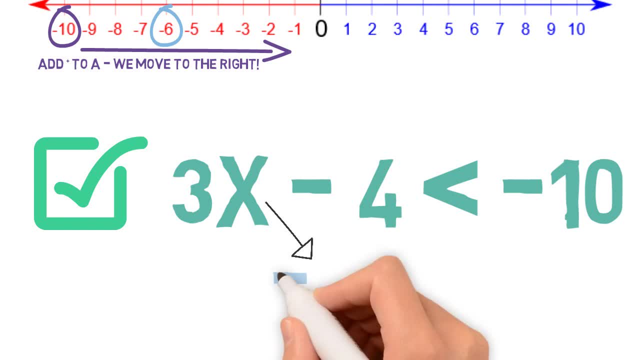 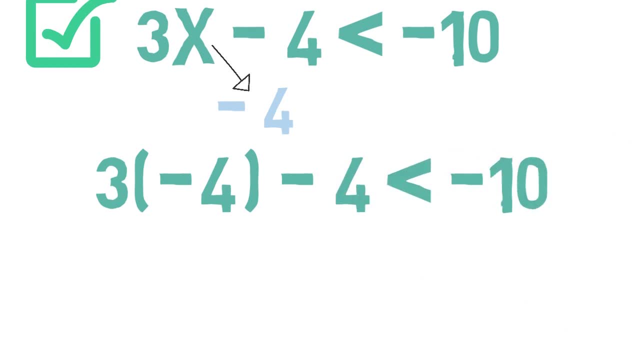 to divide 3x by 3. We have: 3x minus 4 is less than negative 10.. I'm going to replace x with negative 4.. So 3 times negative 4 minus 4 needs to be less than negative 10 for our solution set. 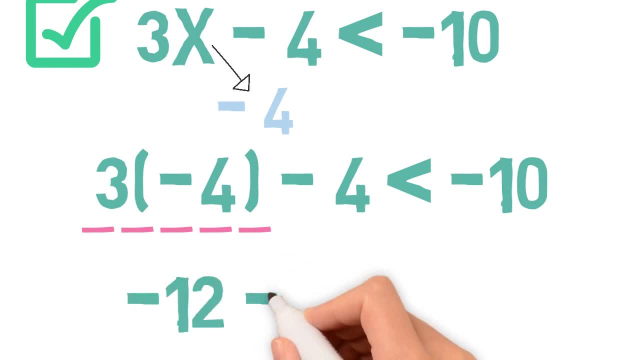 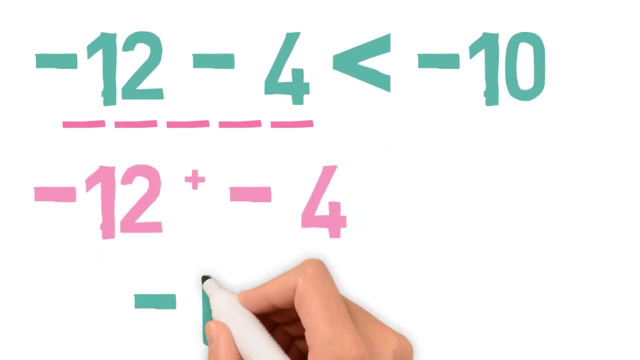 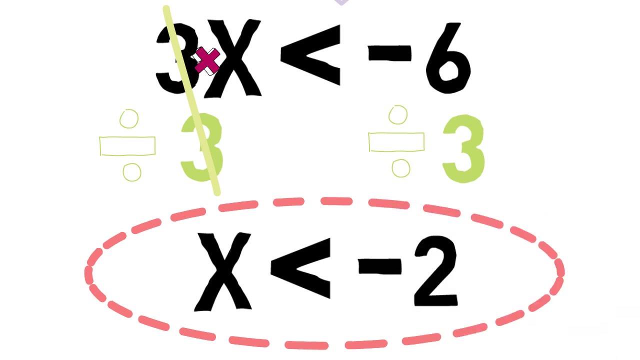 to be true. 3 times negative 4 equals negative 12.. Negative 12 minus 4 is the same thing as negative 12 plus a negative 4, which equals negative 16.. Negative 16 is less than negative 10.. So our solution set of x being less than negative 2 works Way to go. You just solved a two-step inequality.